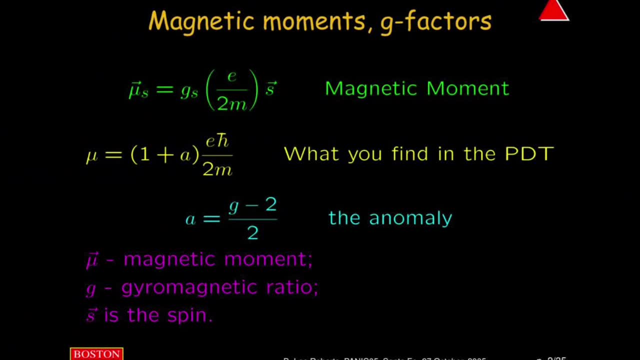 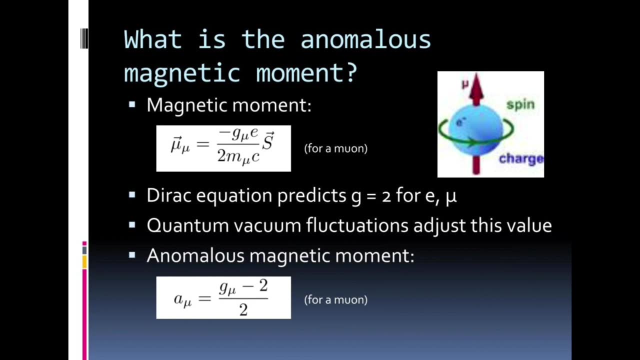 help scientists understand some of the universe's unsolved mysteries, such as dark matter or the reason behind the mass of the Higgs boson. Recent measurements from the muon g-2 experiment at Fermilab have corroborated previous results, increasing the precision of the muon's magnetic 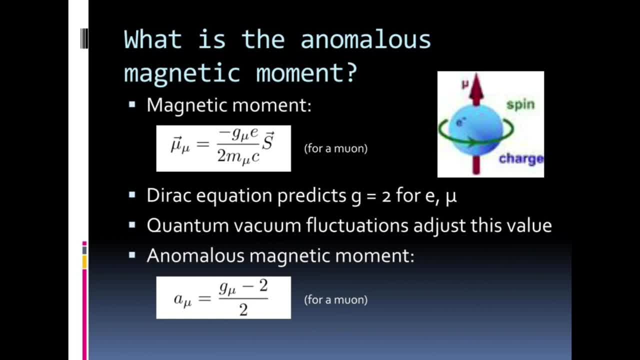 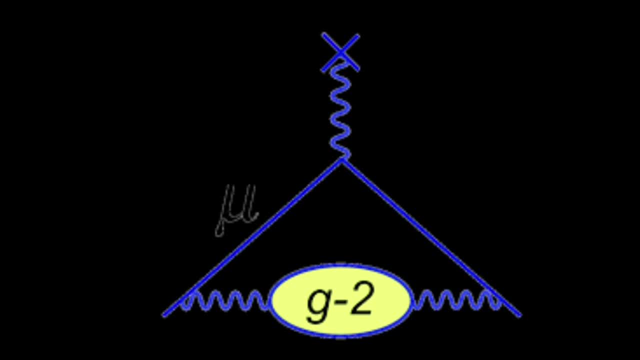 moment measurement to an error of just one part in 5 million. This has strengthened the case that the anomaly is real and not a statistical fluke or an experimental error. The resolution of the muon anomaly lies in either refining the standard model's predictions or discovering new particles that could explain the discrepancy. 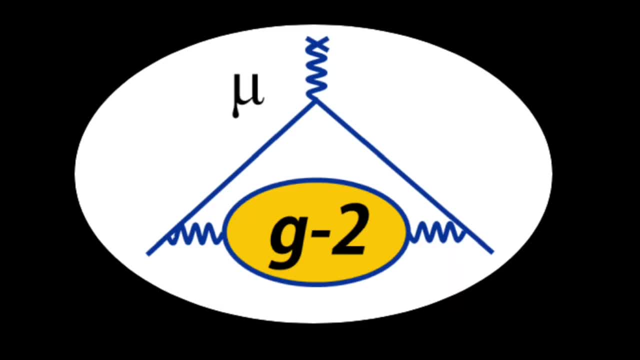 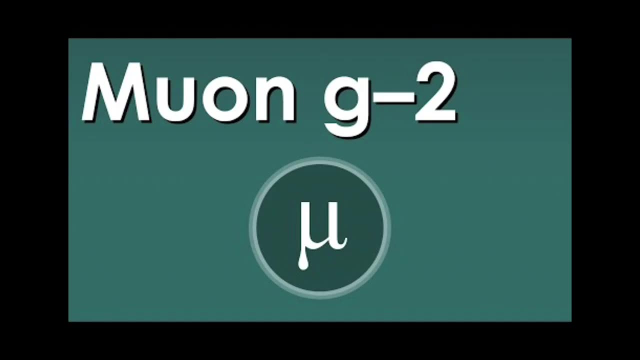 Theoretical physicists have proposed various extensions to the standard model, including supersymmetry and dark photons, which could account for the anomaly. The muon g-2 anomaly remains one of the most intriguing puzzles in modern physics. As experimental techniques more refined and theoretical models more sophisticated, the scientific community moves. 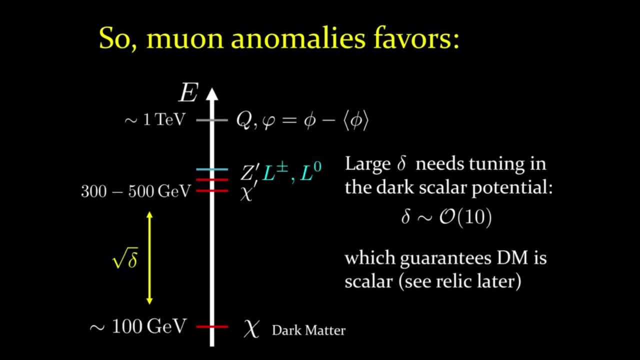 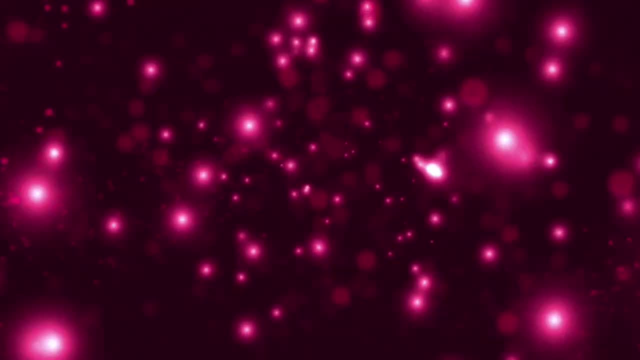 closer to resolving this anomaly. Whether it leads to a confirmation of the standard model or to new physics, the journey of understanding the muon anomaly continues to captivate physicists around the world. 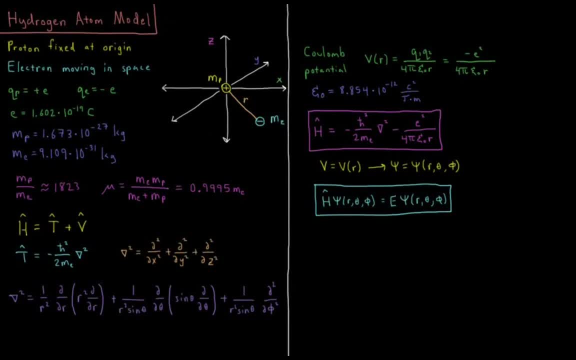 This video will discuss our fourth quantum mechanical model system, the hydrogen atom. So for our hydrogen atom model we have two particles. We have a proton of mass mp, We have an electron of mass me. The distance from the proton to the electron is this value, r. So our 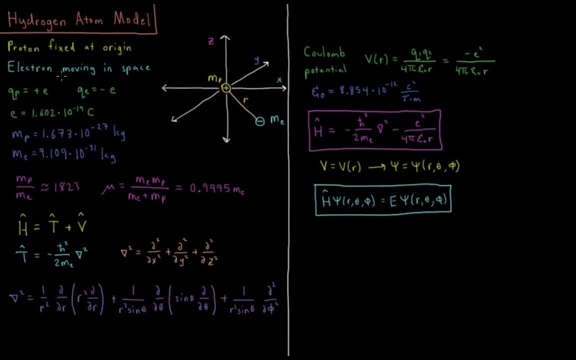 proton is going to be fixed at the origin and our electron is free to move anywhere in three dimensional space, in x, y and z. The charge of our proton is plus e and the charge of our electron is minus e, e being the magnitude of the charge of the electron 1.602 times 10 to the 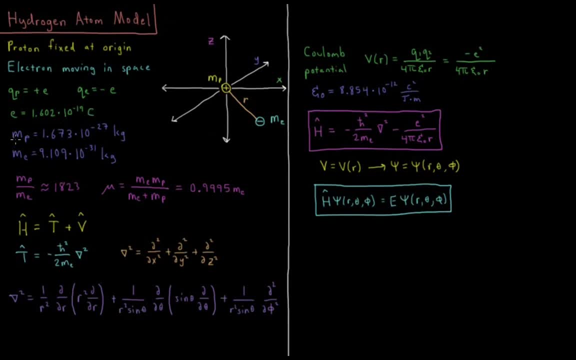 19th coulombs. in SI units, Mass of the proton is 1.673 times 10 to the minus 27 kilograms. Mass of the electron is about 2,000 times smaller than that, being 9.109 times 10 to the minus 31 kilograms. So, as I said, the ratio of the mass of the proton to the mass of